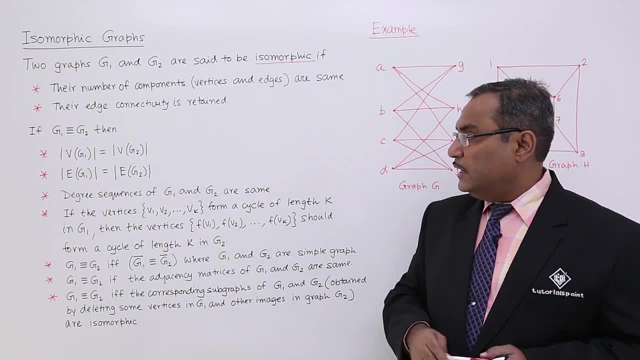 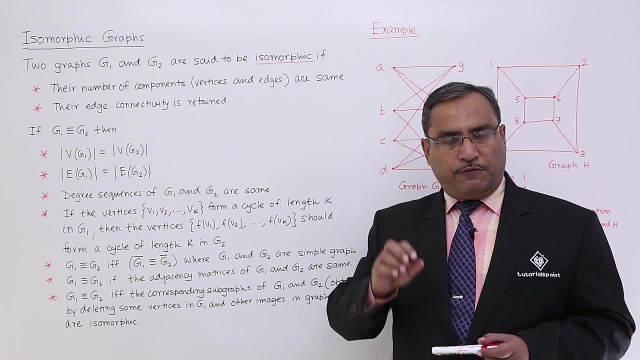 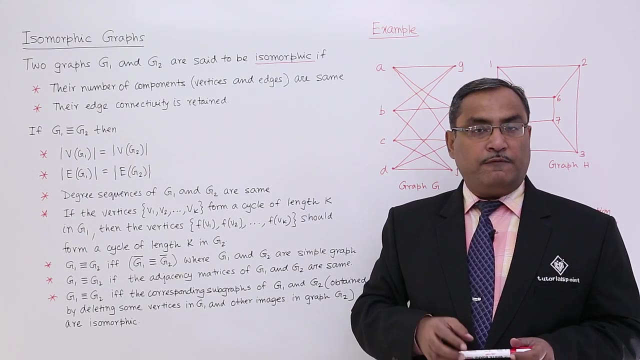 of G2. that also we have discussed in the previous definition. Degree sequences of G1 and G2 are same. We know that number of edges falling to a certain or connected with a certain node will be denoted, will be the count will be denoted by degree for that very particular. 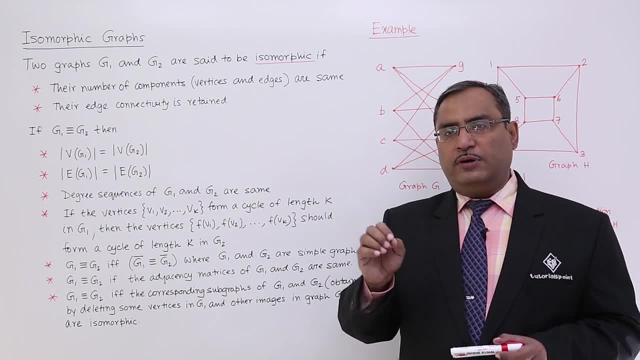 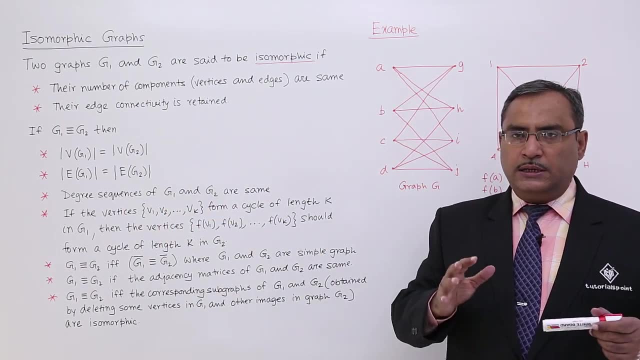 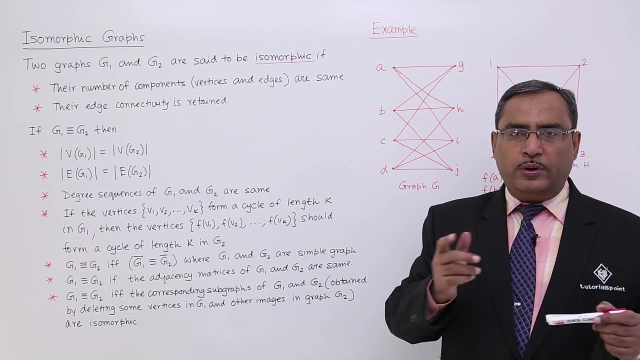 node or vertex. That means number of edges connected to a vertex will be known as a degree of the vertex. So degree sequences of G1 and G2 must be same. That means the we will be having the corresponding image vertices on G2 corresponding to G1, where the degree values 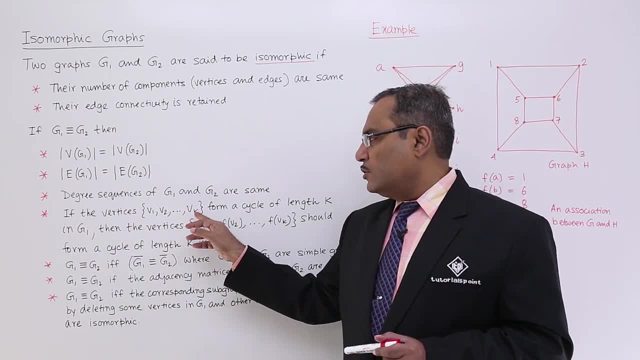 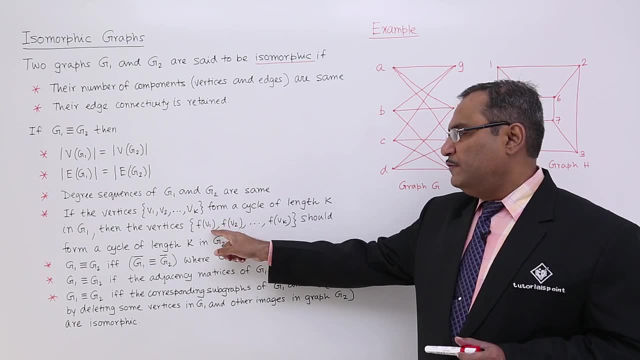 will remain the same. If the vertices V1, V2, dot dot dot Vk from form a cycle of length k in G1, then the vertices f of V1, comma f of V2, dot dot dot f of Vk should form a. 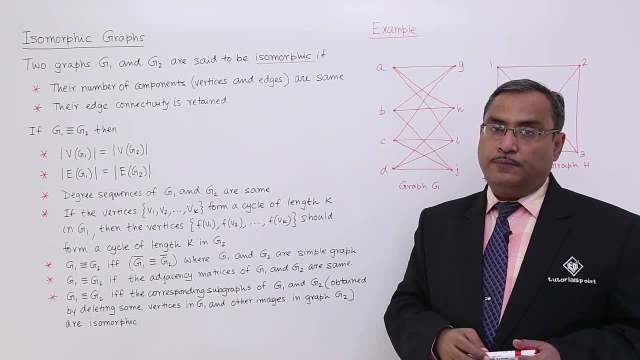 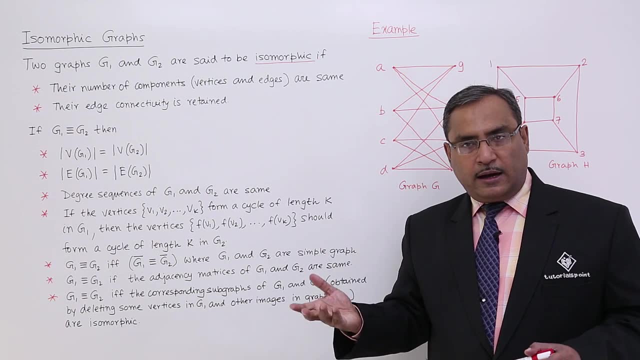 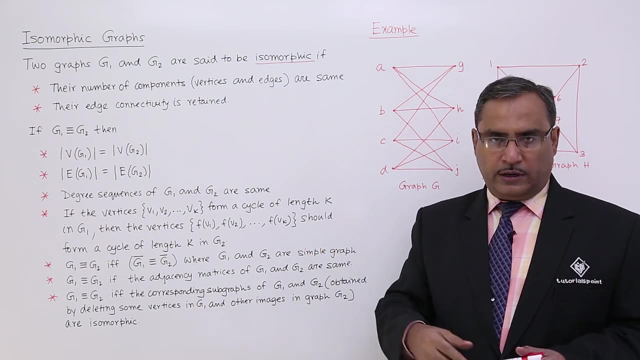 cycle of length k in G2 also. So if that is a cycle of length k in one graph, then there will be cycle with length k in another graph, in the respective, with the respective vertices. If it is V1 here, then in the other graph it is f of V1.. 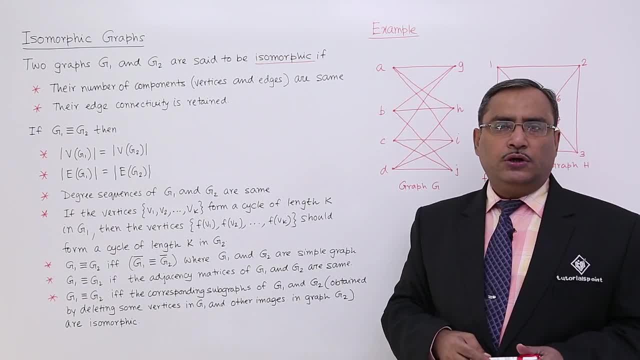 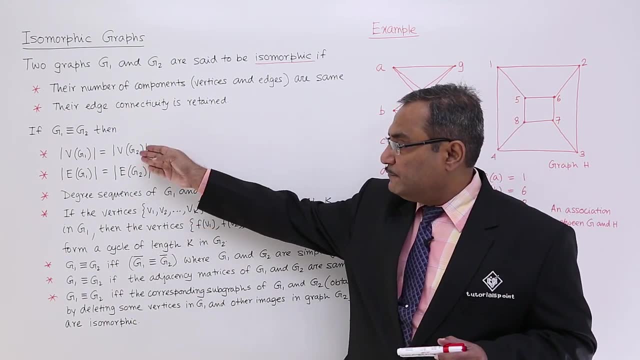 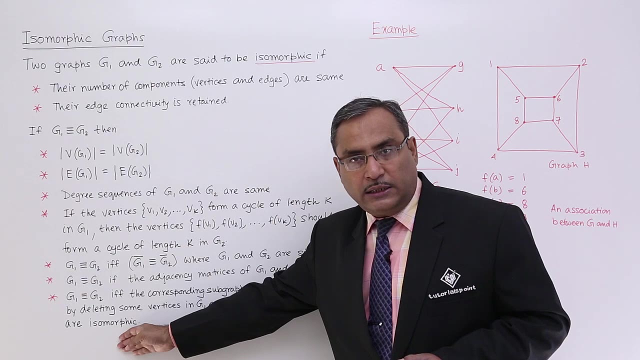 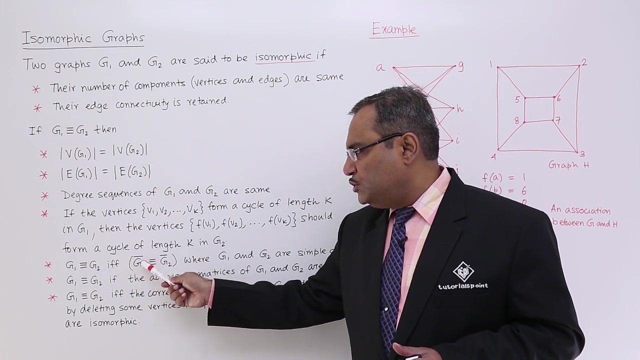 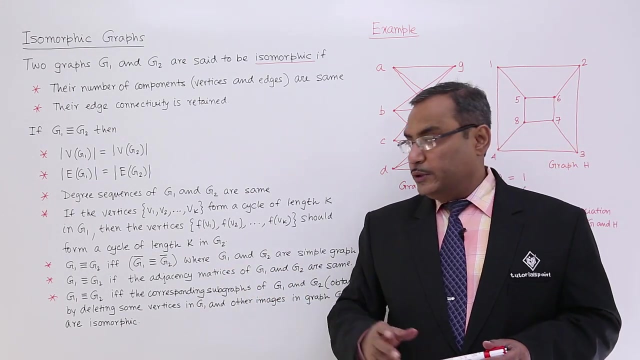 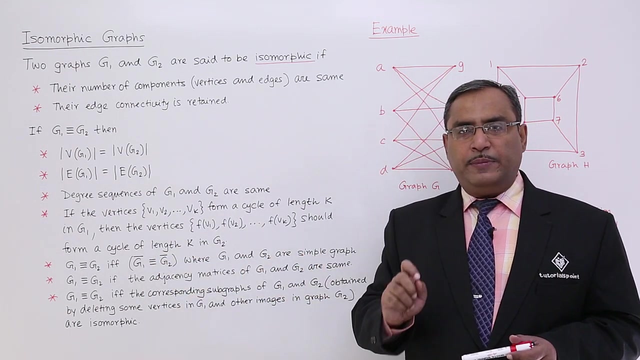 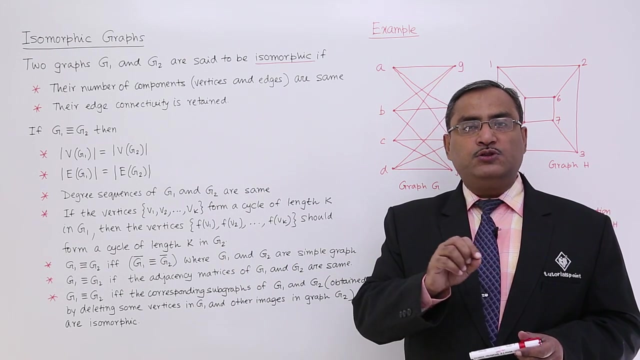 We have used two terminologies: one is a complement, another one is a simple. We know the simple graph is that graph which is having no parallel edge or no loop. And complement of a graph means in G1, if there is one edge between V1 and V2, then in G2 there will be no edge in. 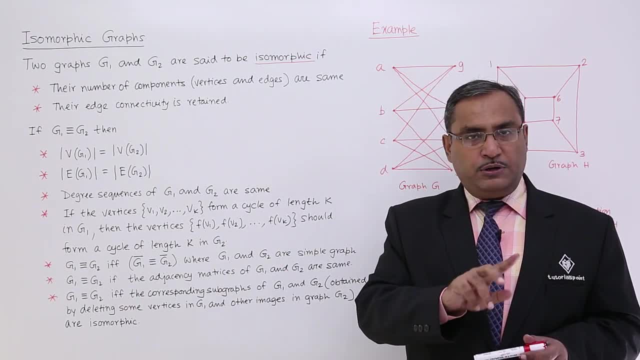 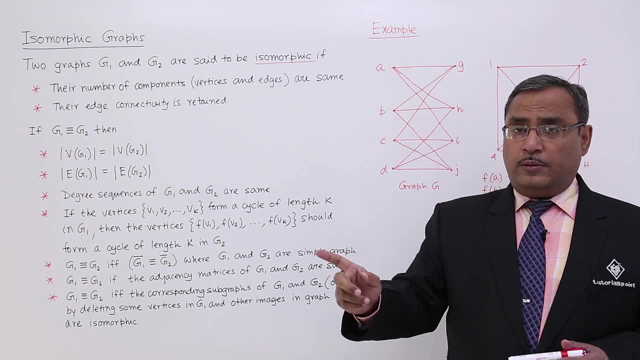 between V1 and V2.. In G1, if there is no edge in between V1 and V2 through vertices, then in G2 there will be one edge between V1 and V2.. Not V1 and V2, the respective vertices. 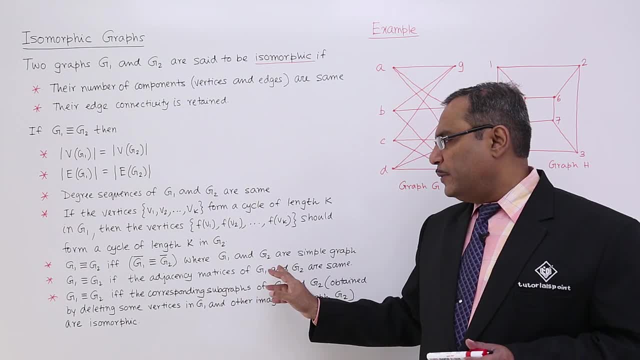 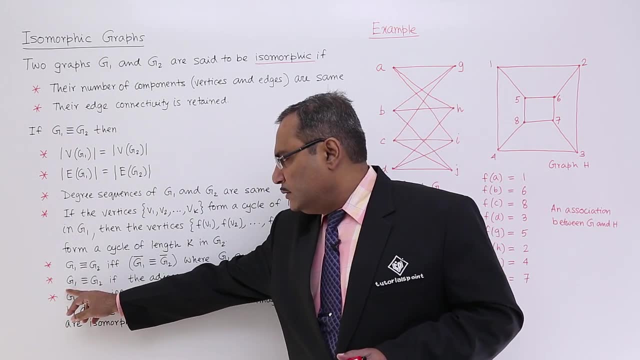 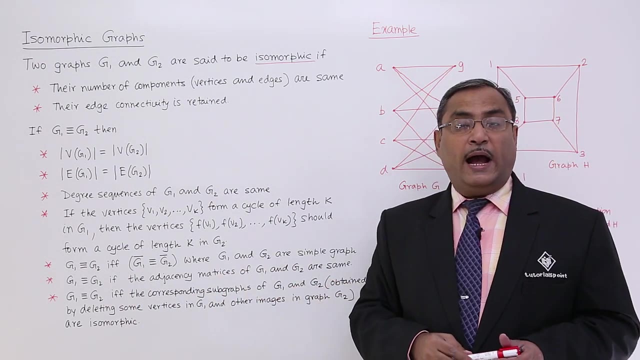 So that is known as a complement. We are having a separate video on the how to calculate the complement of a graph. please watch that one also. Y, f, G1 is isomorphic to G2 if the adjacency matrices of G1 and G2 are same, So accordance matrices. 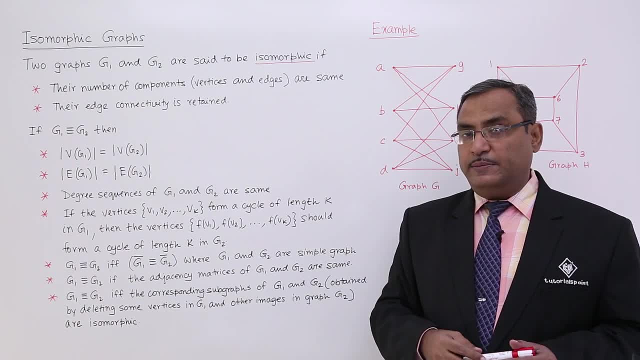 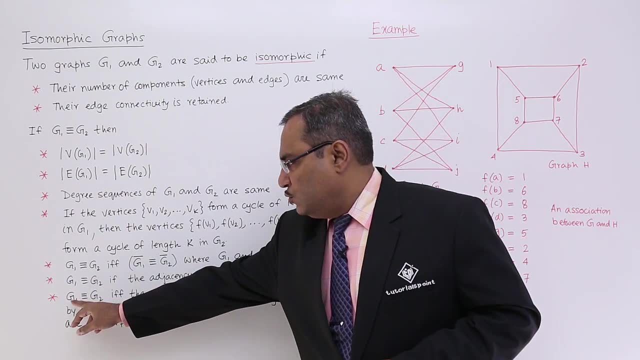 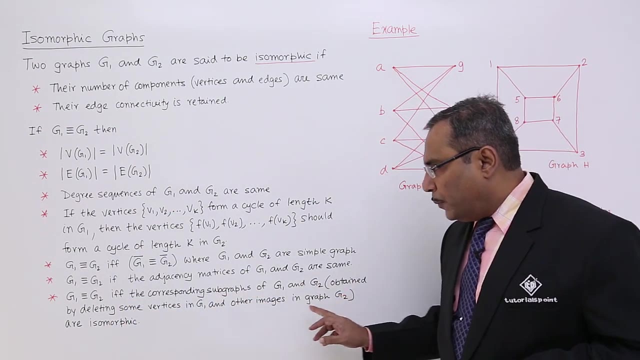 must be same. We know that. what is adjacency matrix, how to represent a graph through the adjacency matrix. We have having an separate video on that also. So G1 is isomorphic to if, and only if, the corresponding subgraphs of G 1 and G 2, obtained by deleting some vertices. 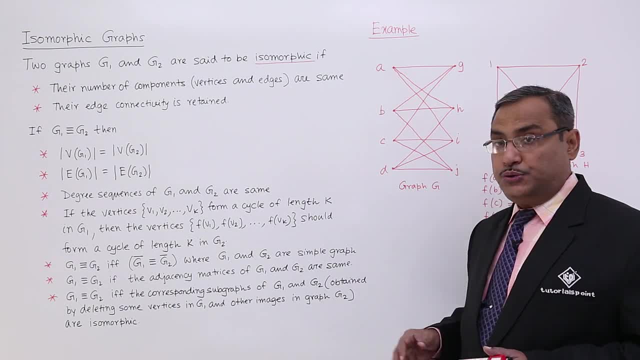 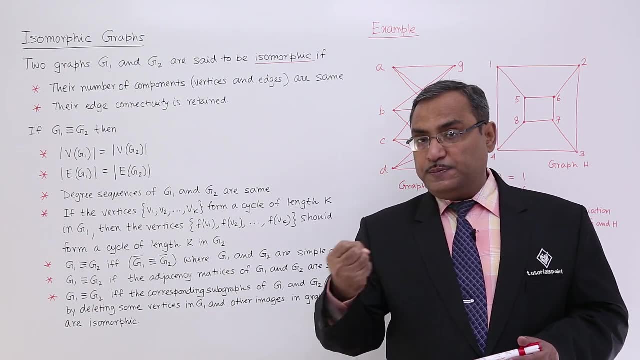 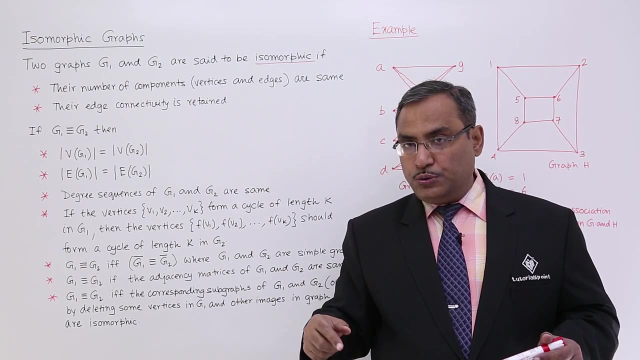 in G 1 and other images in graph G 2.. That means if you take a subgraph from G 1 and then if you take the respective image vertices from G 2, that means we are getting two subgraphs from G 1 and G 2 with the vertices V 1 to V k, say, and with the vertices F of V 1 to. 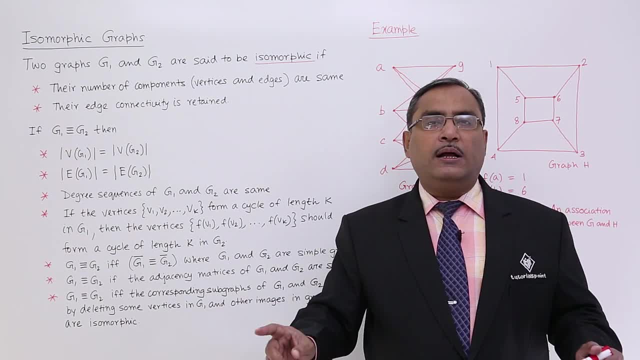 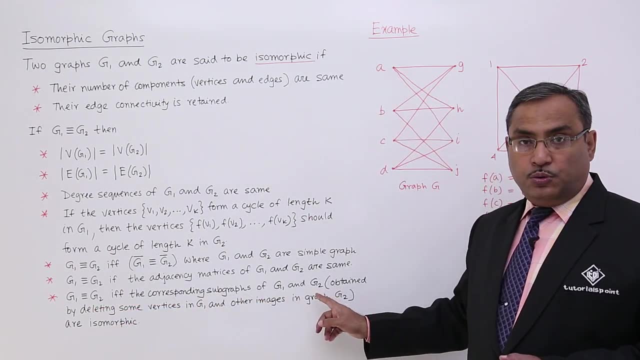 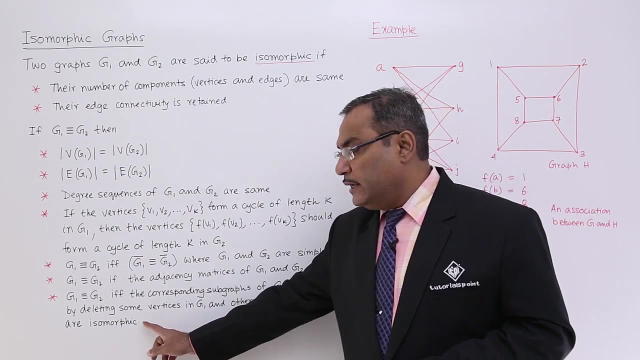 F of V, k say. In those cases these two subgraphs must be also isomorphic. So this particular subgraphs of G 1 and G 2 will be obtained by deleting some vertices in G 1 and some and other images in graph G 2, and they must be isomorphic. So these are the next subgraphs. 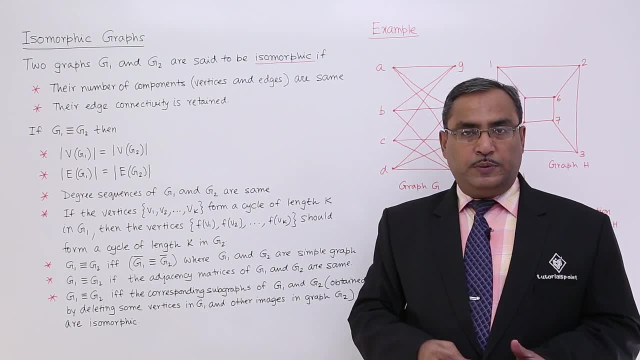 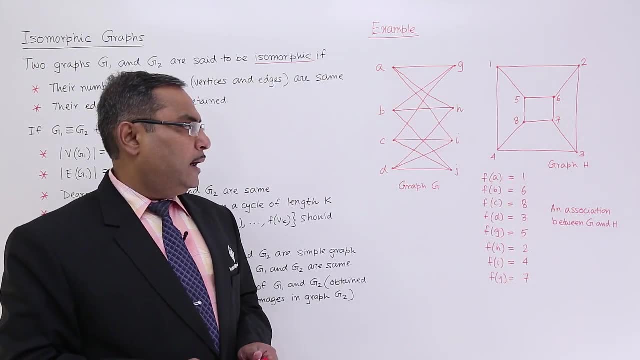 necessary and sufficient conditions between the two graphs to be said that they are isomorphic. We cannot miss any one of them. So, as an example, consider this very two graphs: One graph is G, another graph is H, So this is one graph. You see, here we are having vertices. 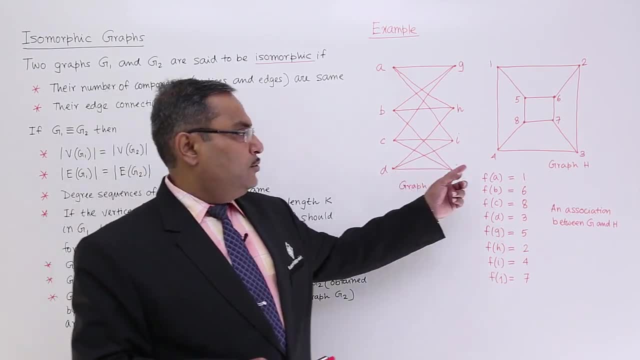 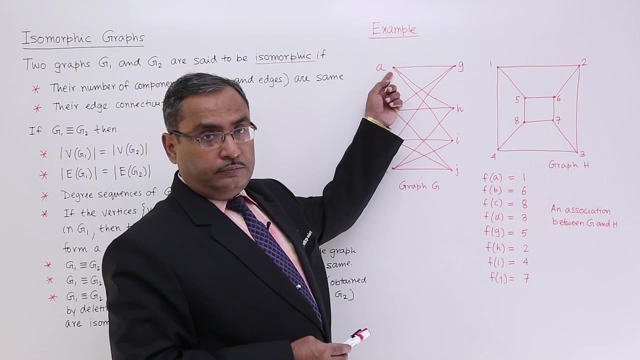 like A, B, C, D and then G, H, I, J. Here we are having the vertices like 1, 2, 3, 4,, 5,, 6,, 7, 8.. So now see, A is having degree 3 and then 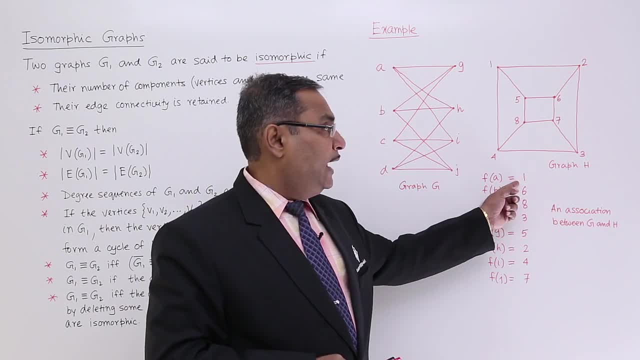 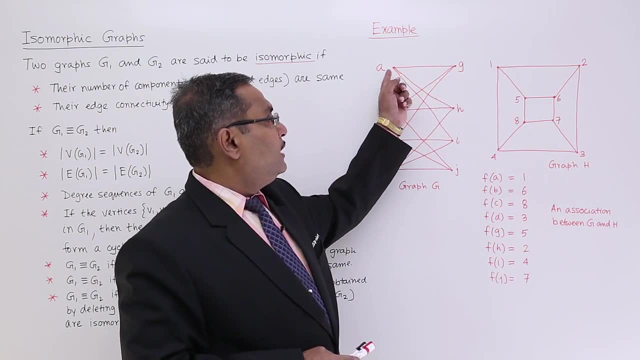 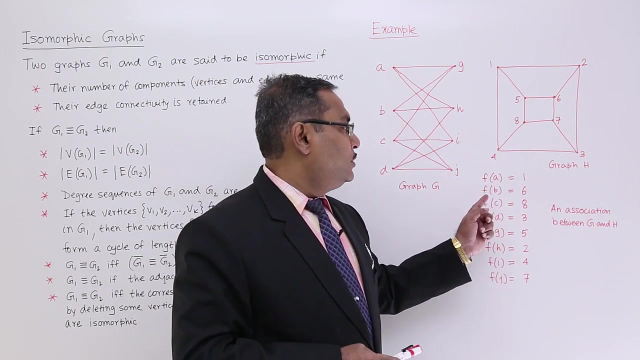 corresponding, the image vertex in H will be having the 1 and that is also having the degree 3.. And if you go for the connectivities, if you go for the connectivities, A is connected with G, A is connected with H and A is connected with I. So now A, here, 1, 1 is connected. 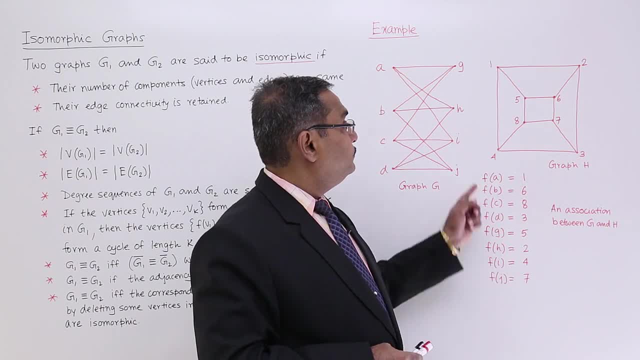 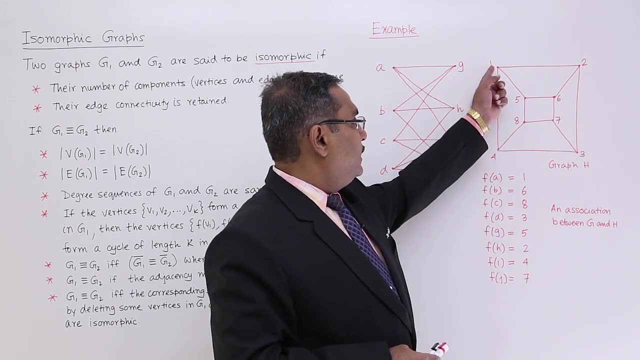 with 2,. 2 stands for H, So this one. Next, 1 is connected with 5.. So 5 means G. Now this one, and 1 is connected with 4.. 4 stands for I. That means A is connected with I. So